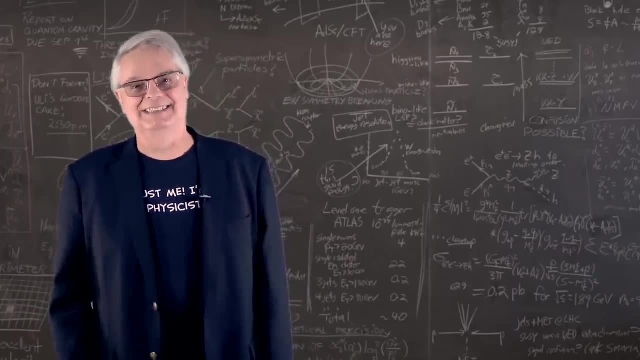 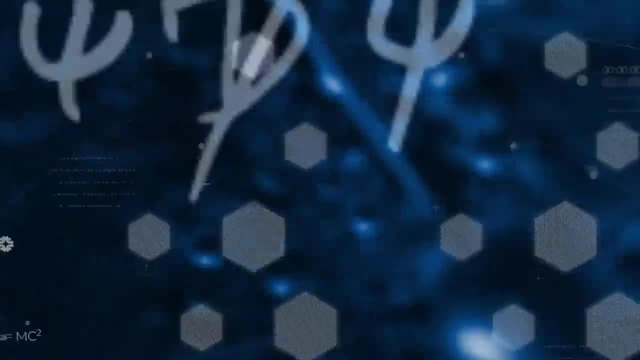 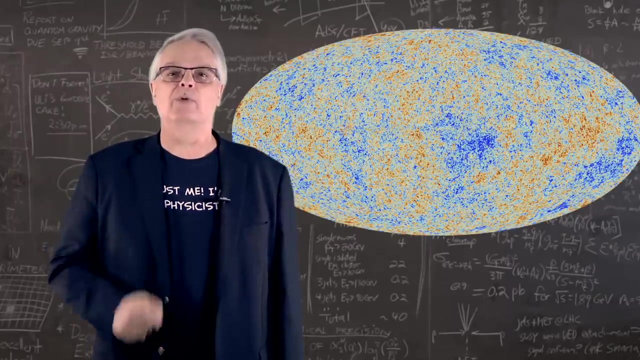 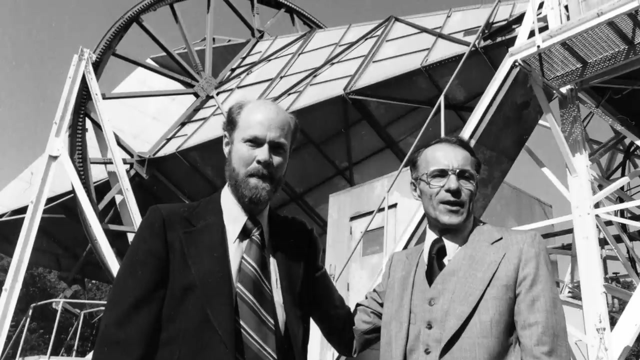 trove of information about the universe, So let's look into it. The Cosmic Microwave Background Radiation, or CMB, is the earliest thing we can see in the history of the cosmos. It was discovered in 1964, and it represents a time when the universe cooled. 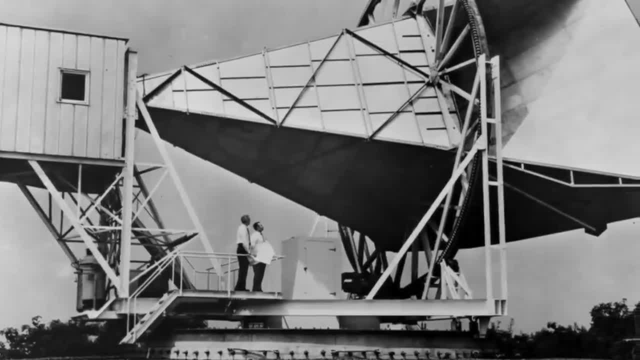 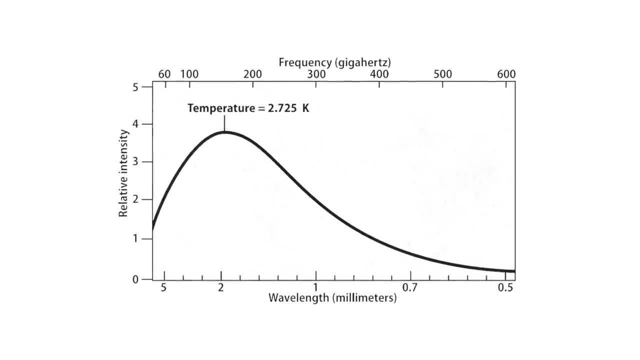 enough to be transparent a mere 380,000 years after the universe began. Because of the expansion of the universe from then until the present day, the temperature of the afterglow of the Big Bang is now higher than ever before. The cosmic microwave background radiation, or CMB, is 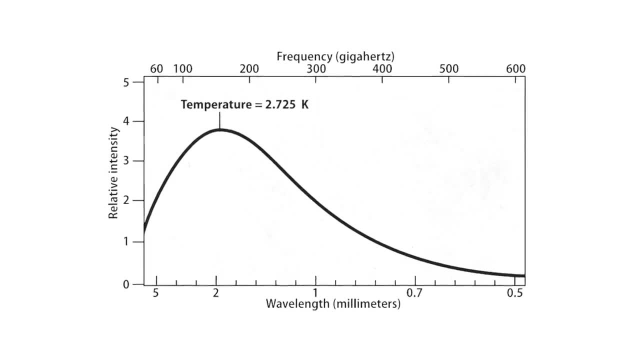 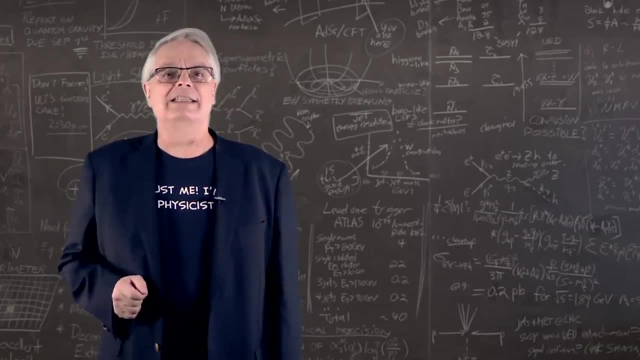 now 2.7 Kelvin, or minus 450 degrees below zero Fahrenheit. That temperature is the same in every direction. Indeed, the CMB is a sphere around us. However, to represent that sphere here on the screen, we need to make it two-dimensional. That's done in the same way this map of the Earth is. 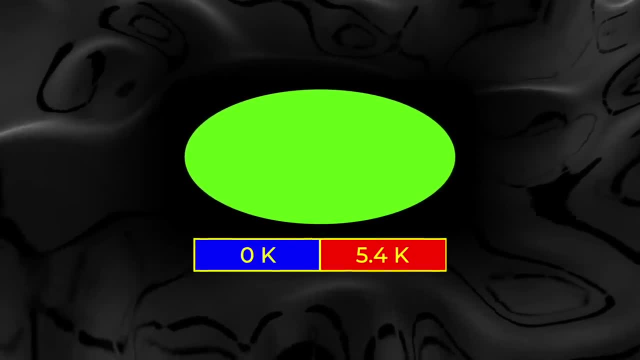 done. So what you see here is a representation of the CMB as seen from Earth. Red is 5.4 Kelvin and red is 5.4 Kelvin. So what you see here is a representation of the CMB as seen from. 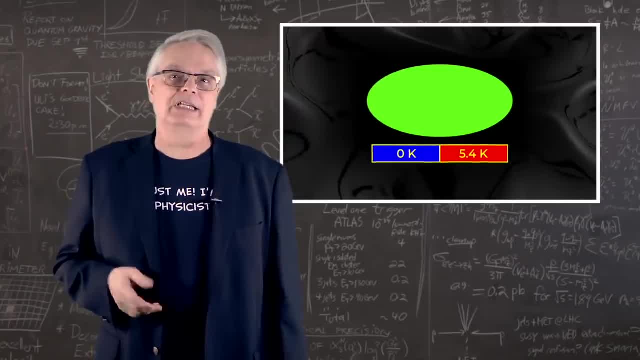 Earth. Red is 5.4 Kelvin and red is 5.4 Kelvin. So what you see here is a representation of the CMB as seen from Earth. Red is 5.4 Kelvin and blue is 0 Kelvin. Of course, you don't see either red or 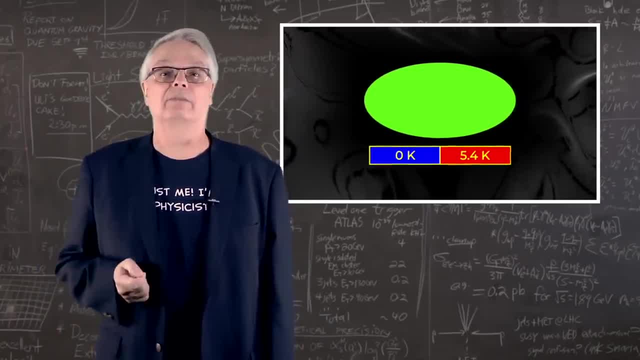 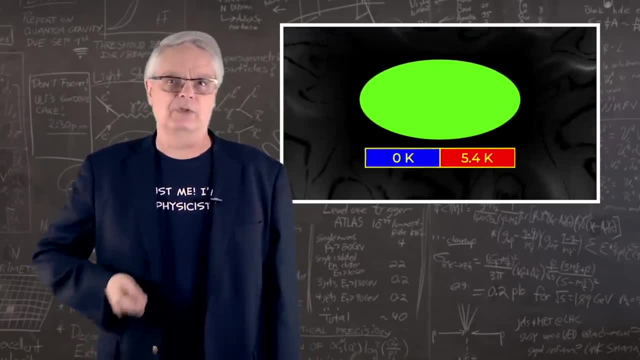 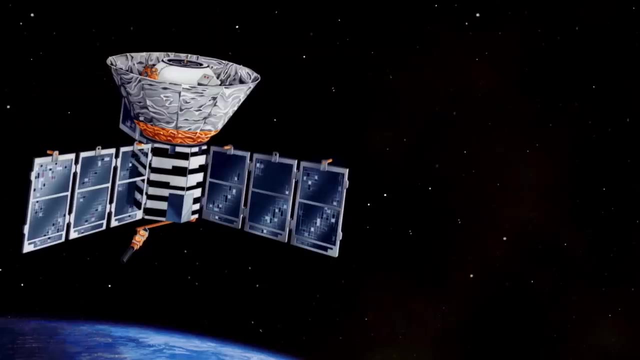 blue. all you see is green, which represents 2.73 Kelvin. The reason it's green everywhere is the CMB is the same in every direction to within about a tenth of a percent. The measurement was made much more precisely in 1998 when a satellite called the Cosmic. 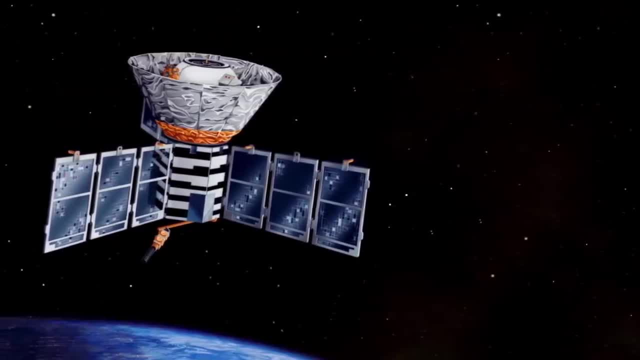 Background Explorer, or COBE, looked for tiny variations in the CMB. When researchers looked at the data, they found that the CMB was the same in every direction. So what you see here is a representation of the CMB as seen from Earth. Red is 5.4 Kelvin and blue is 0 Kelvin. Of course, 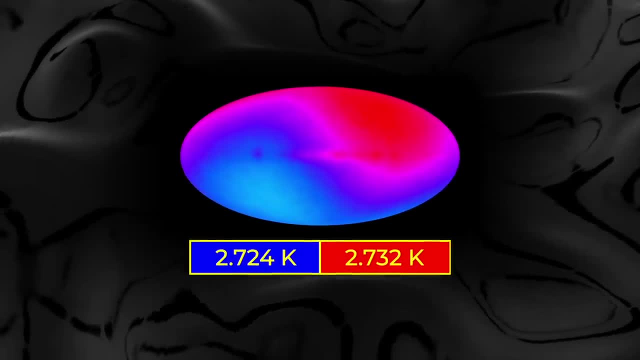 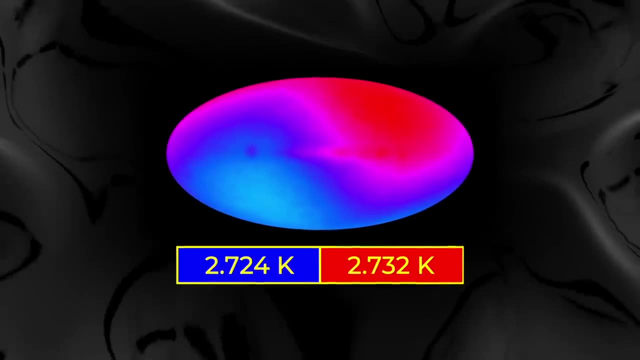 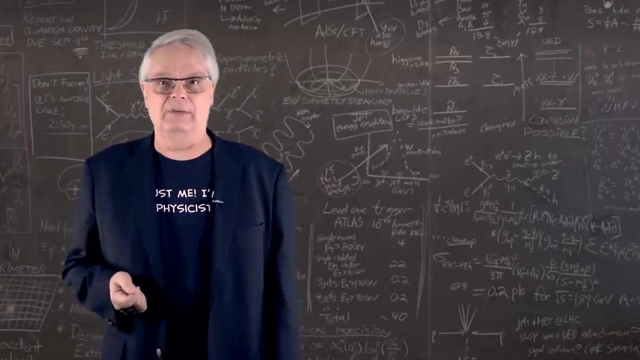 they saw that half of the sky was a little hotter than the other, with one side being 2.724 and the other side being 2.732 Kelvin. What's that all about? Well, the simple existence of the CMB told the biggest story, which is that the Big Bang happened. This little non-uniformity is because 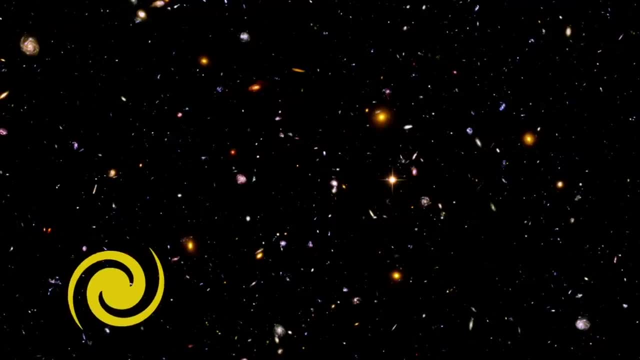 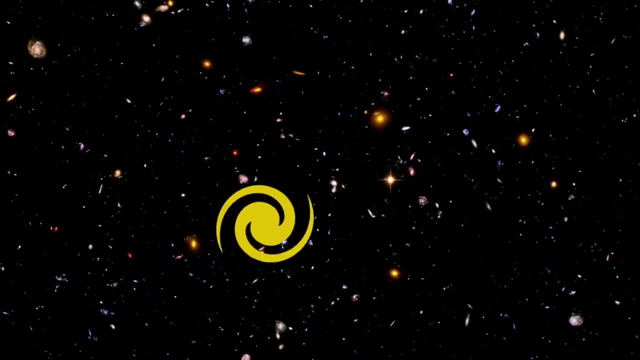 the Earth is moving. with respect to the CMB, It's the same basic idea as the Doppler shift that astronomers use in the CMB. So what you see here is a representation of the CMB as seen from the CMB, To tell us that galaxies are effectively moving away from us, except this tiny shift. tells us that, compared to the average velocity of the universe, the Milky Way is moving about 370 kilometers per second in the direction of the constellation Leo. Once we understand that the Milky Way is moving compared to the average of the rest of the universe, we can subtract off that. 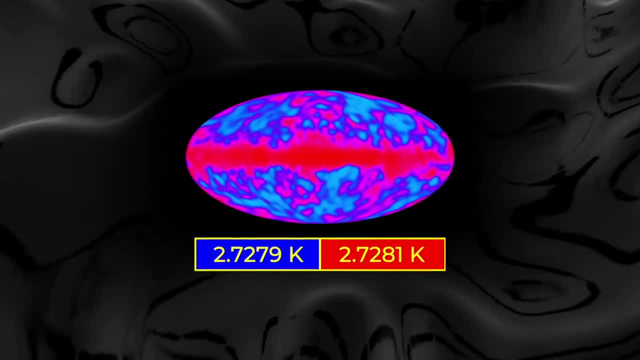 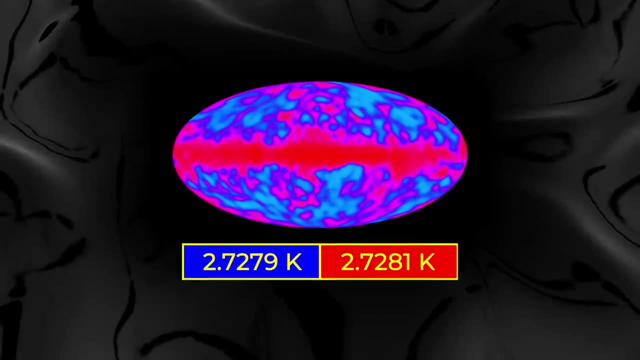 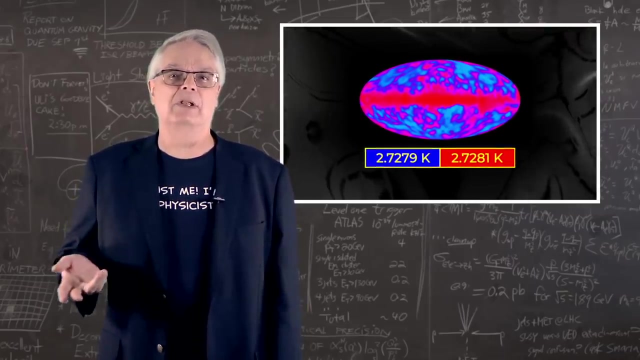 effect and look for even smaller variations. Now the differences in temperature between red and blue that you see here are only 200 microkelvin, and we see this red stripe across the equator. That red stripe is caused by microwaves emitted by gas in the Milky Way and we have to subtract. 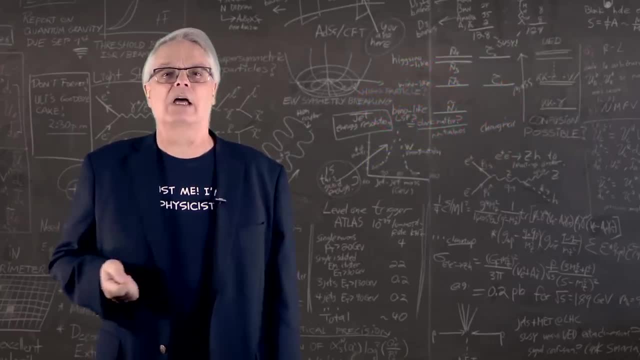 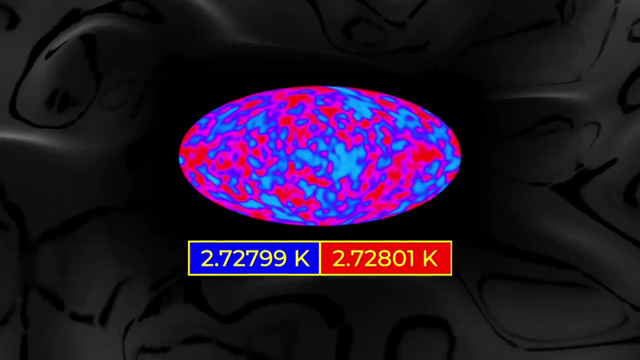 that off too. When the COBE astronomers erased the contribution from the Milky Way, they were left with this red and blue splotchy picture, which is a precise measurement of the tiny non-uniformities in the CMB: The temperature difference between the red 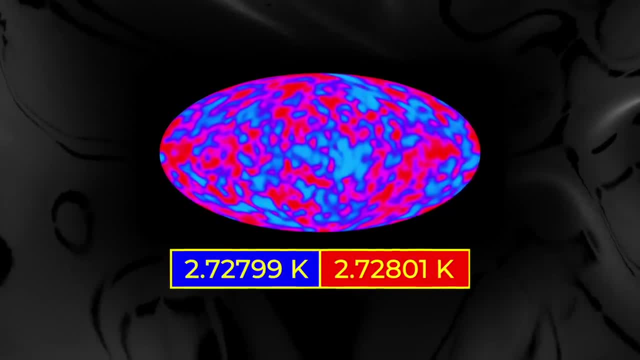 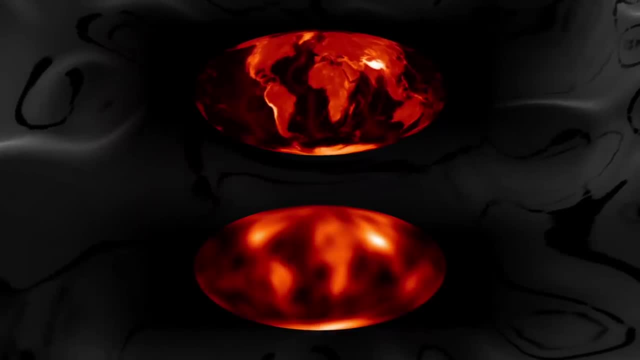 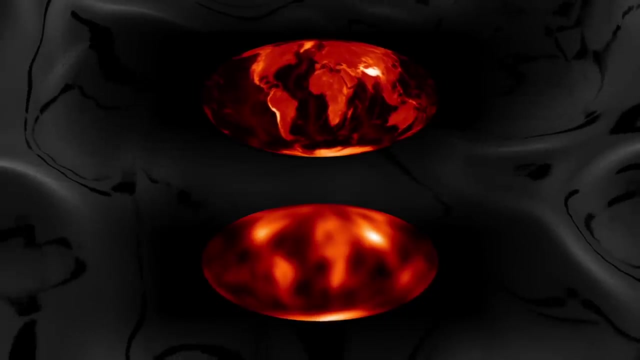 and blue spots in this picture is only about 20 microkelvin. This was a huge accomplishment, but we need to give some context. Here is a picture of the Earth and what that same picture would be like if it were photographed by the COBE satellite and that photograph were processed. 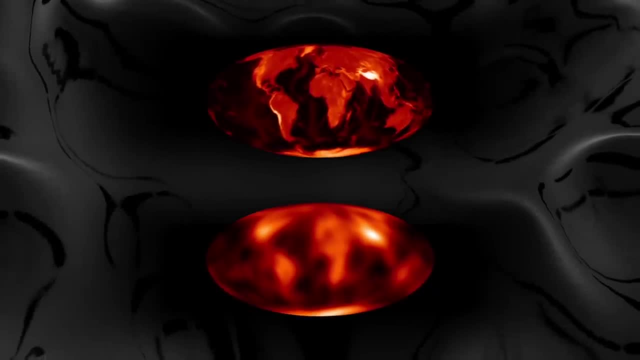 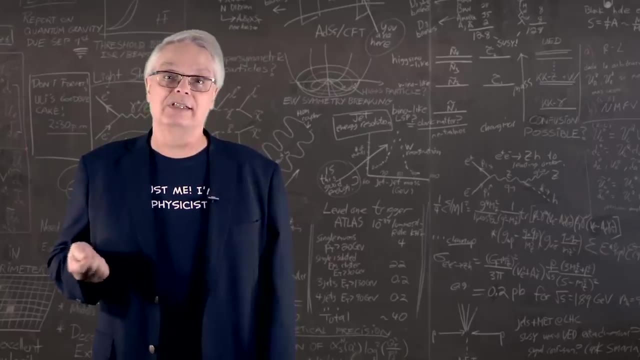 through the COBE algorithms. You see it's pretty blurry. Now, this shouldn't be thought of as a criticism. The COBE result is already 20 years old and the technology used in the satellite was older than that. However, there have been two other satellites launched in the intervening time. 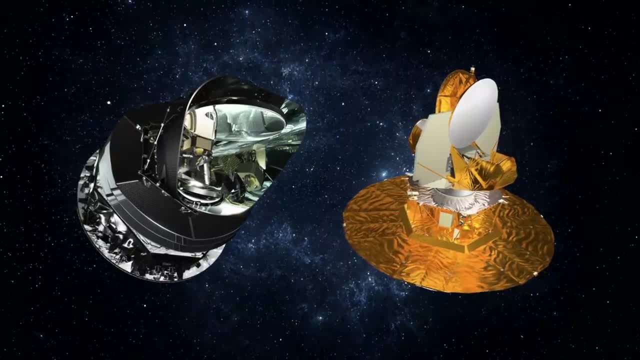 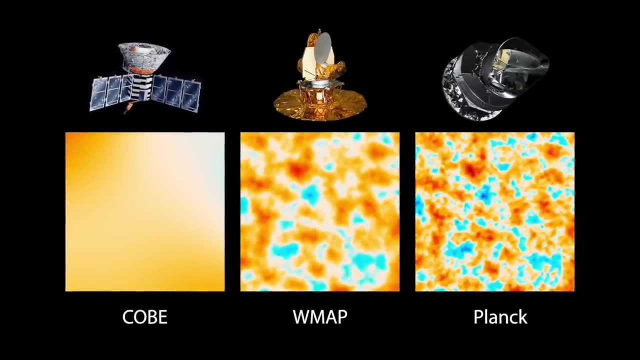 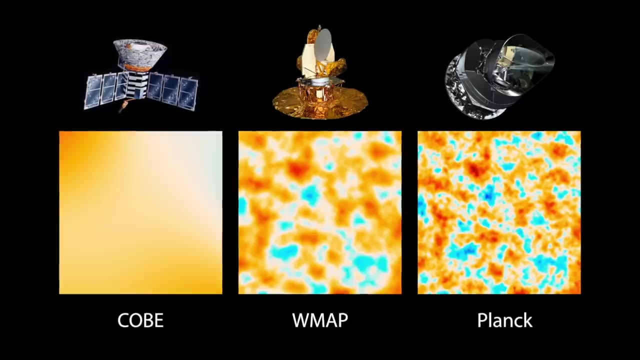 one called WMAP in 2001, and one called PLANC launched in 2009.. As you can see here, each instrument was able to image the CMB with improved precision, and the PLANC satellite gets the best image of the CMB. This is simply a treasure trove of information. There's a lot. 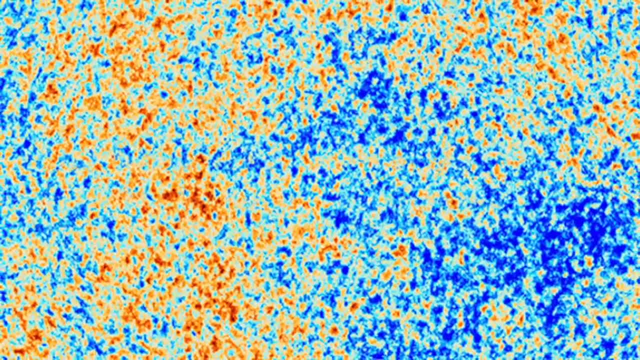 of science. in them there spots. Those spots reflect sound waves that were present in the universe when it was 3,000 years ago. The PLANC satellite was able to image the CMB with improved precision and the COBE satellite was able to model the CMB with improved precision and the PLANC 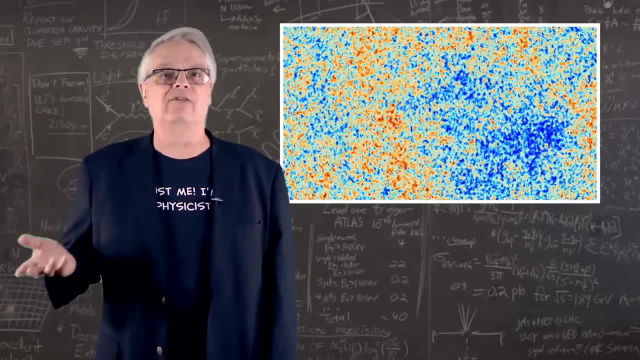 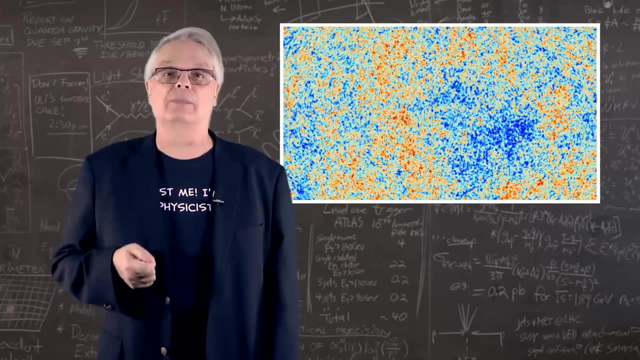 satellite was able to use it to measure. the CMB Sound is just density variation in a material, in this case the plasma of the early Big Bang. The reddish-orange spots are locations where the plasma was denser and the bluish spots were where it was less dense. Now it turns out to 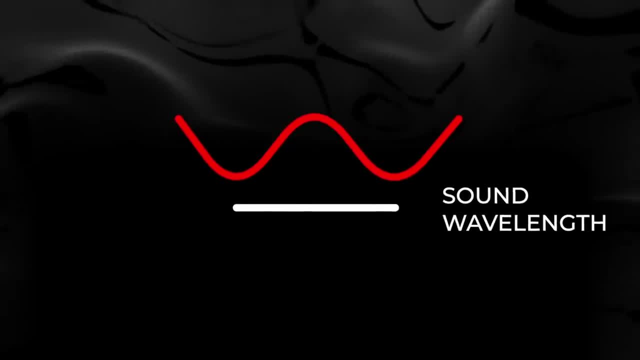 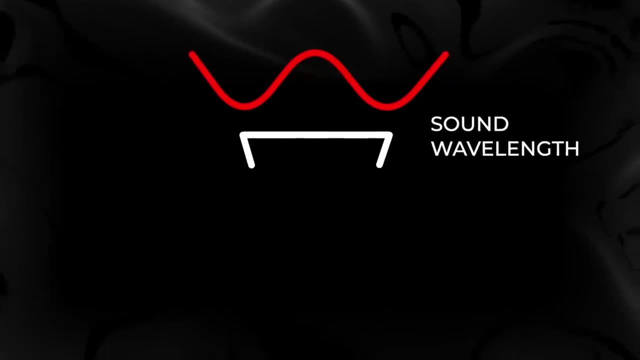 not be super hard to calculate the most common wavelengths that could develop in the Big Bang's hot plasma before the CMB became visible. Furthermore, we know how far away the sphere that holds the CMB from the CLB will be. So if the SAMS of the CMB became visible, the CLB would. 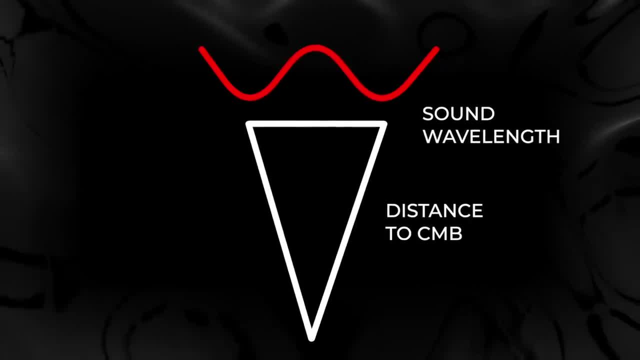 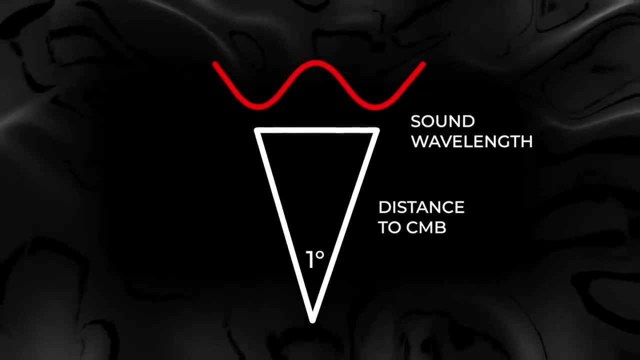 be more visible. So if the SAMS of the CMB became visible, the CLB would be more visible. So if the CMB is in the present day, Those two distances set up a triangle and astronomers can calculate what should be the most common angle between adjacent hotspots. It turns out to be about 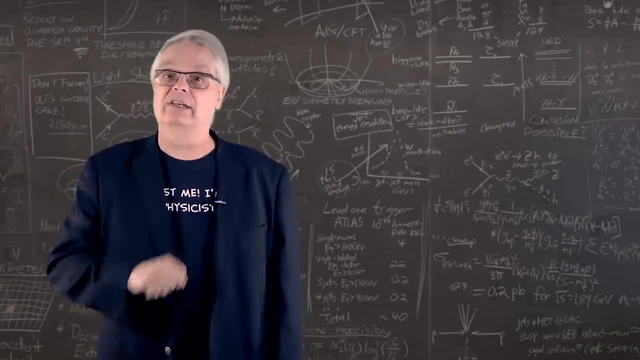 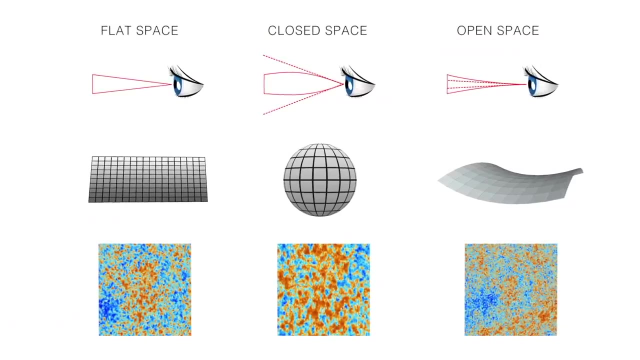 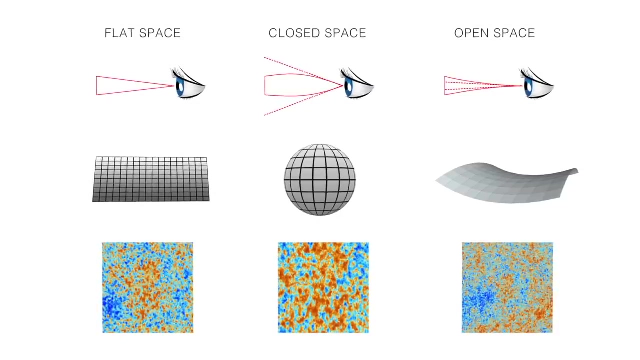 one degree, But hold on. That's if space is flat. If space is curved in some way, say like a sphere or a saddle, then the lines connecting the CMB in our eyes will be distorted. That will make the apparent angle different from what happens in flat space, and it will 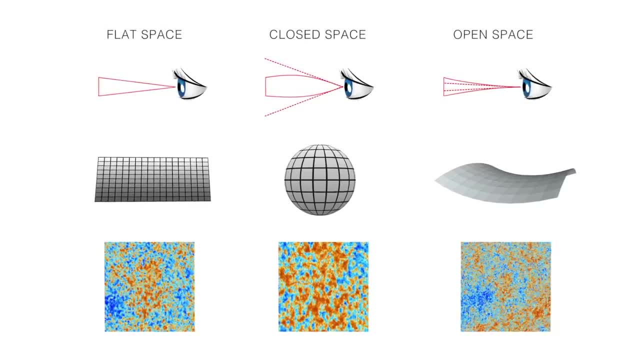 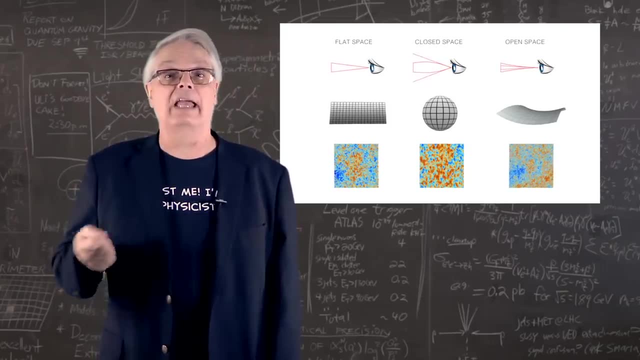 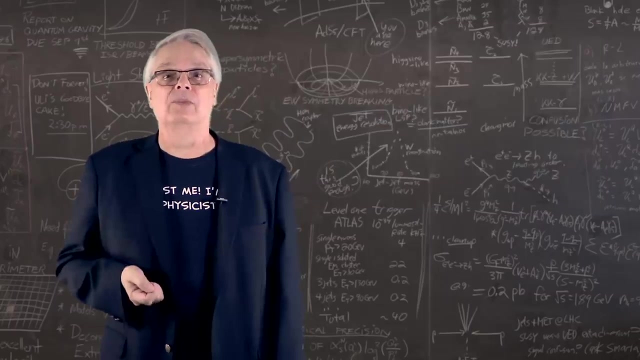 change the distance we see between adjacent spots: Bigger if space is spherical and smaller if space is saddle shaped. That means measuring the angular distance between adjacent spots is a good way to determine the flatness of space. So if we look at the Planck data we can determine the most common angle between bright. 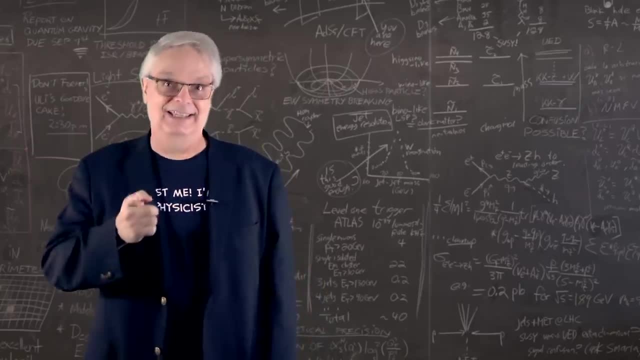 spots. and what do we see? A drum roll, please. It's about one degree. We can see that here. The CMB is in the present day. It turns out to be about one degree. We can see that here, The CMB is in the present day. It turns out to be about one degree. We can see that here. 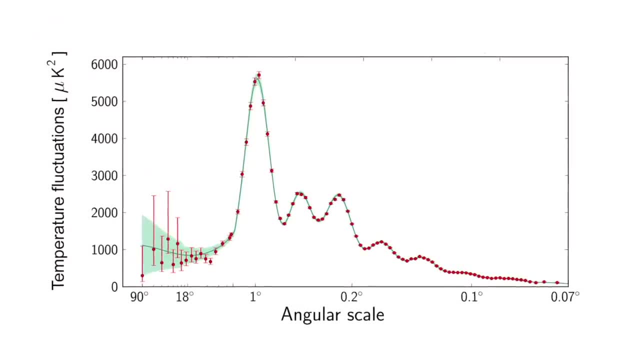 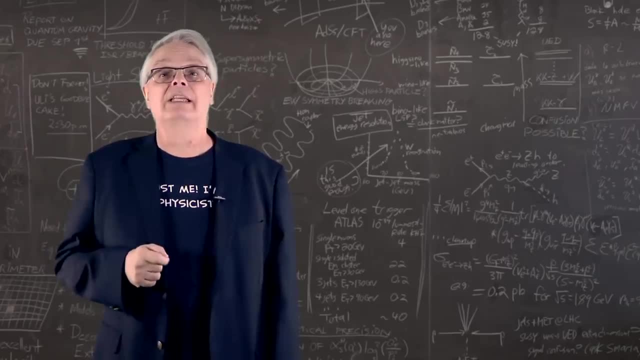 We can see that here. The CMB is in data and the line is a fit and the peak is at about one degree. So that means that space is flat, or nearly so. However, this is an experimental measurement, which means that the one degree number isn't infinitely precise. It has an 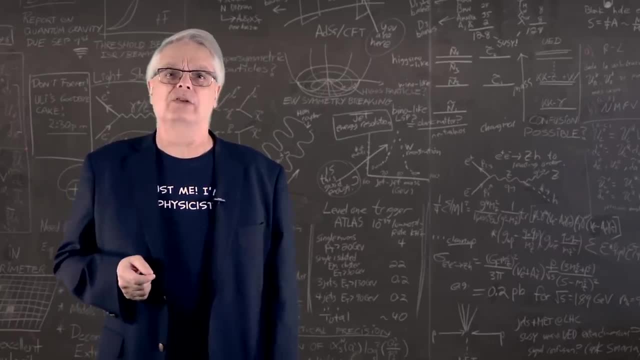 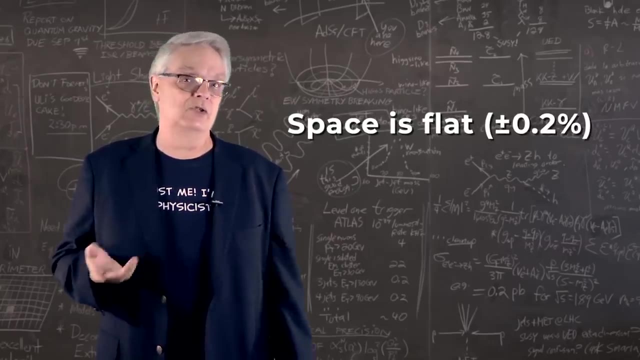 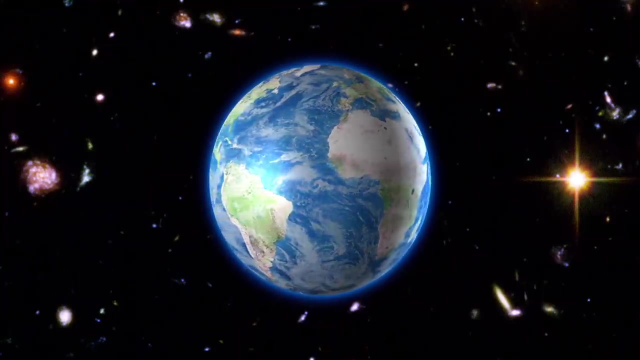 uncertainty associated with it. If you take that uncertainty, you can say that while flat space is most likely, the uncertainty allows at most a curvature of space of about 0.2 percent. This maximum curvature of 0.2% means that the universe is bigger than we can see with the total universe. 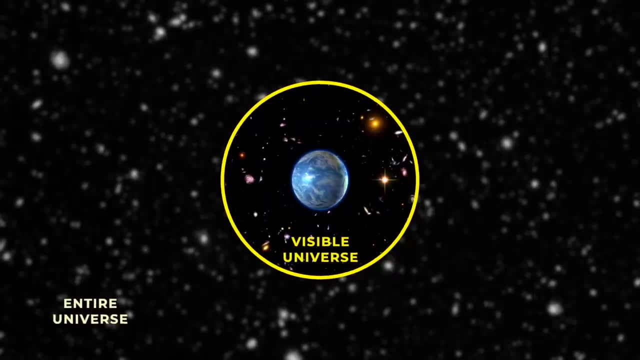 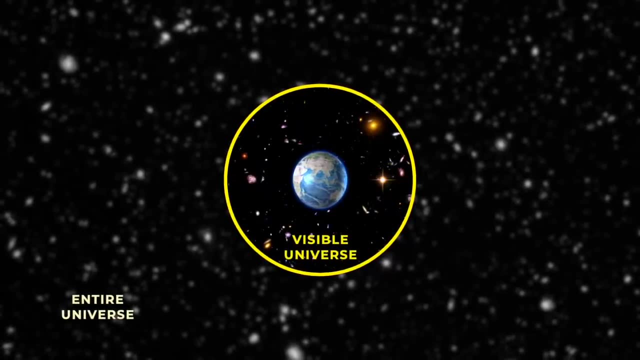 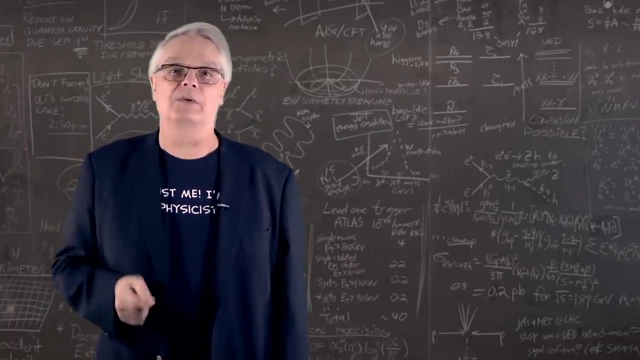 having a radius of at least 500 times bigger than the visible universe, And that means that the volume of the entire universe is at least 125 million times bigger than the universe we can see. It could be even bigger, And all that information can be determined just by looking at these tiny.